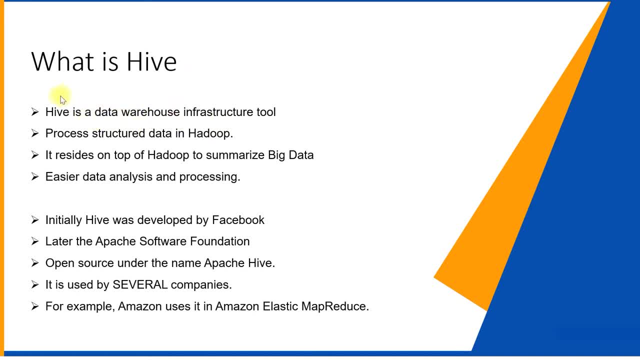 the primary purpose. You create the data warehousing solution in Hive database to process only the structured data. in Hadoop, Hive supports only structured data, but if you go with HBase and other technologies they process Semi and then you know other types of data. So Hive is all about structured data. It is 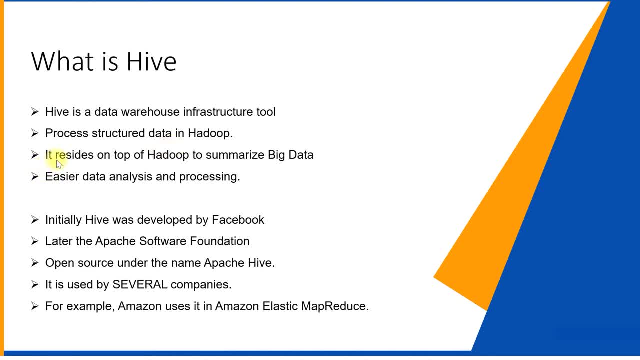 very much similar to any other databases like SQL or SQL Server, but with the exception of having Hadoop HDFS in the background. It leverages Hadoop to perform all the data analysis and processing. So that's why we say that it's always residing on Hadoop And it's easier. 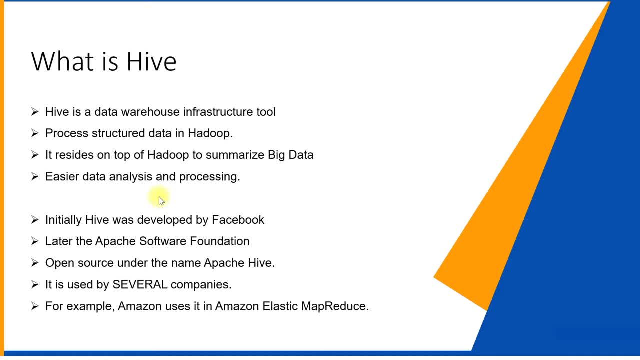 to perform any data analysis and processing, because we're not really writing any MapReduce programs here. It is just about writing a Hive query. We also call it as HQL, So it was initially developed by Facebook for their internal usage, But later on the Apache Software. 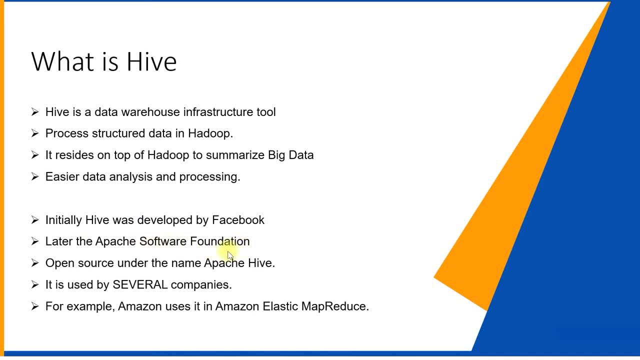 Foundation took it over and it's been developed, you know, in the Apache Foundation and it's currently even it's a open source under the name of Apache hive and it's being used by several companies across the globe. one of the example would be you. 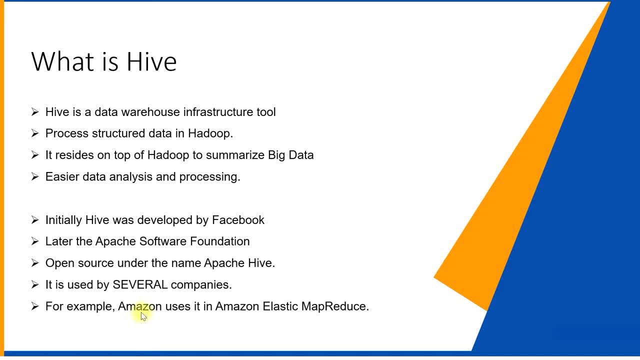 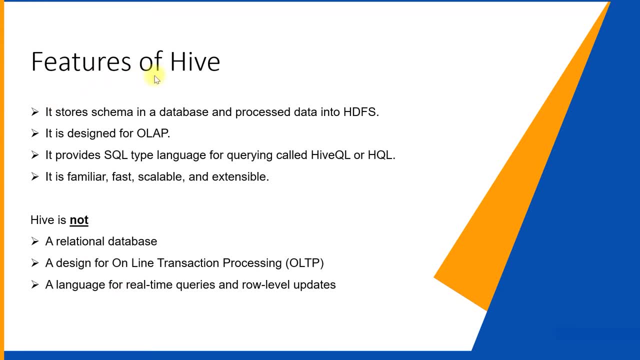 know Amazon, but there are several thousands of companies you know to make use of hive database. now let's look at what are some of the features. right, it stores the schema in a database and processed data into HDFS. so what it means is that it leverages the HDFS concept, like distributed concept, to 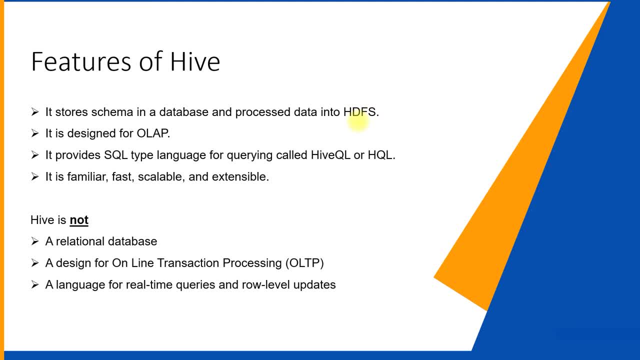 perform any aggregation or any processing of data using the data nodes we will. we'll talk about how it is getting processed. in the next slide, we'll be discussing about architecture, right, so that's how we will be looking into it, and it is designated for OLAP, online transactional processing, like most. 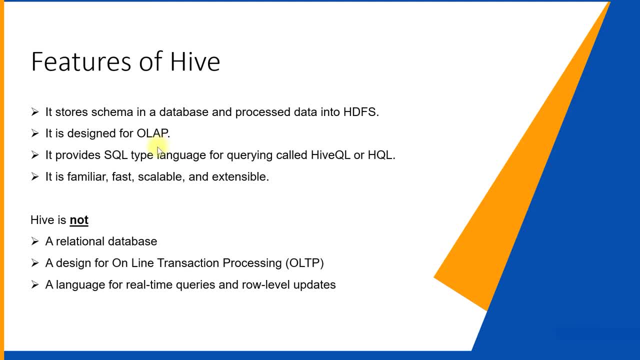 likely. you know right many times where sorry right once and read it many times right. all those OLAP reports are read. you know many multiple times right. so that's why hive is meant for, or designed for, OLAP systems. it provides us equal type of language for querying the data. underneath right it's also called as: 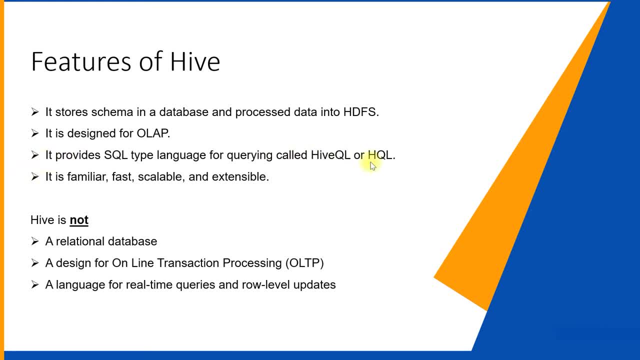 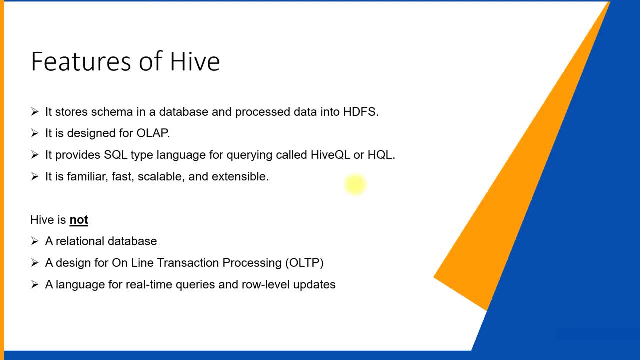 little bit very similar to any my sequel or SQL server, wherein we would be using SELECT star from sovereign table so that internal, internally converted into a MapReduce program in the hive engine like this, also called execution engine. we look at that in the architecture and it's it's a very familiar, fast, scalable or host, then change a比如, because in case 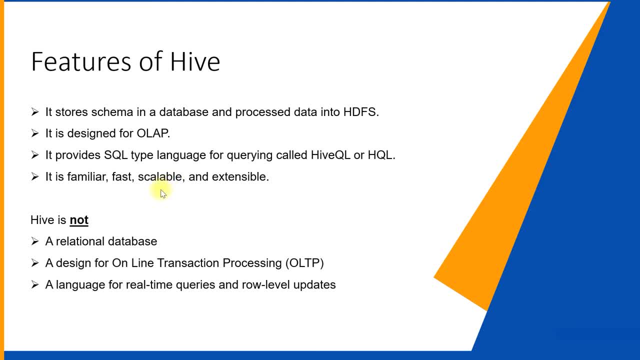 of higher data processing. all we do is you know, expand or scale you are running a certain data sleep vais, are it even available to 현재 or um? so we do, underlying HDFS and your data nodes. that will be very easy because of you know commodity hardwares in the background, right? so that's why we call it a. 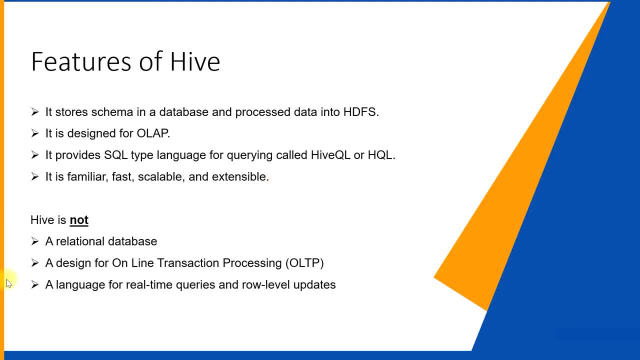 scalable, fast and extensible right. and also there is misconception. misconception especially with hive. hive is not a relational database right, it's not like an Oracle, but wherein it is suitable for OLTP kind of environment right, a language for real-time queries and low-level updates. so this is what. 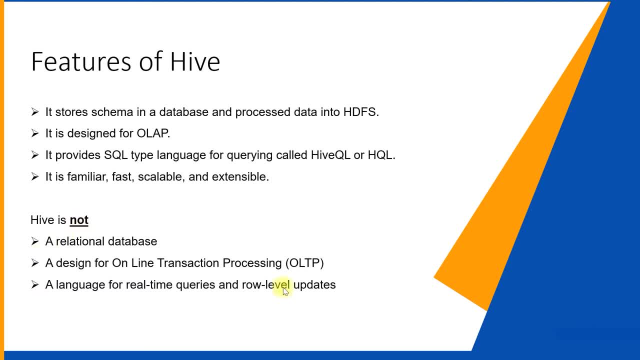 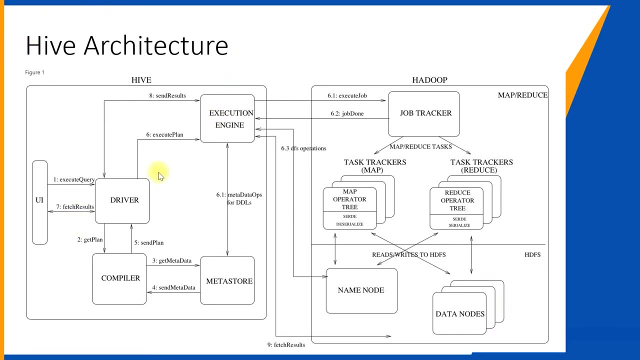 hive is not about right, so we have to be really sure what it is about and what it is not, so that we can make use of hive appropriately in a particular use case. okay, so here is the hive architecture if you look at it. this section, the first. 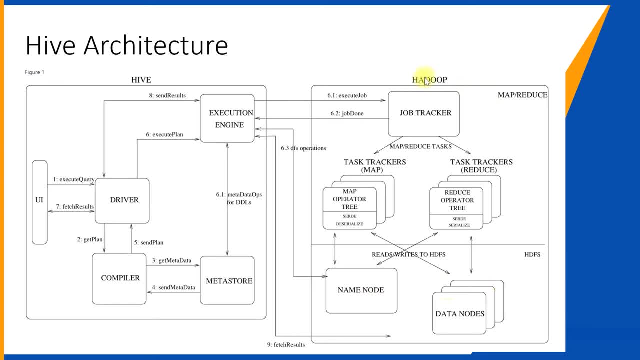 half section is all about hive and the section second section is about Hadoop, right? so typically Hadoop contains: you know, a resource manager, job tracker, right that that works directly with you know, mappers and reducers, and each of those operations connect to name, node and then process the data or any aggregation on. 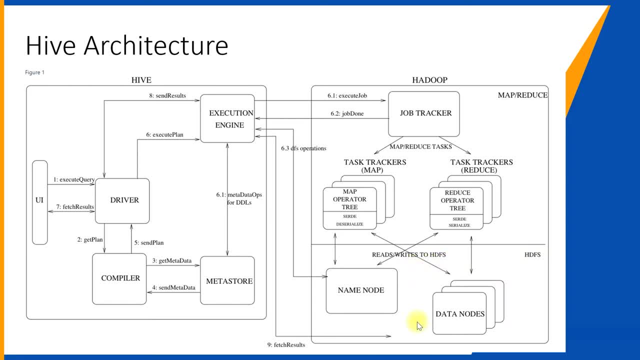 the data nodes: right. all the data processing happens on the data node and name node is something which controls the data node. right. it has the information of what what part of data is in the data node, so that's how you can block is stored on what you know data node- right, so that this is like a master. 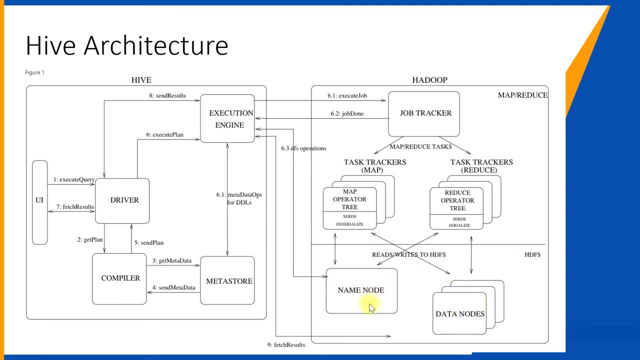 and these are the worker nodes right. so whenever we perform any high query execution, what happens is- if you look at this arrows and the sequence here, the first one from UI- whenever you execute on any high query, it first goes to a driver. a driver is an interface between various components, like you know. 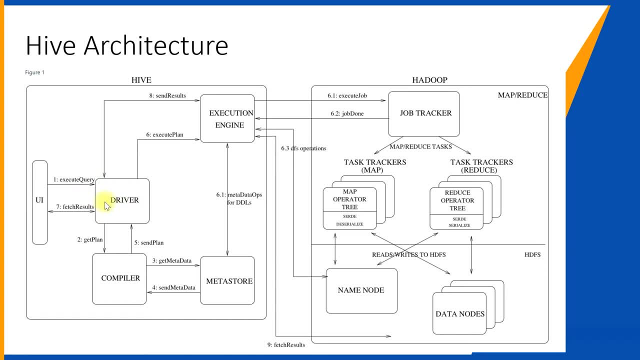 compiler and also execution engine right. it takes that high query and passes to the compiler so that the compiler can actually connect to Metastore and get the information that is required for the execution. so what is a Metastore here? a Metastore is nothing but a metadata about hive itself. so for example, 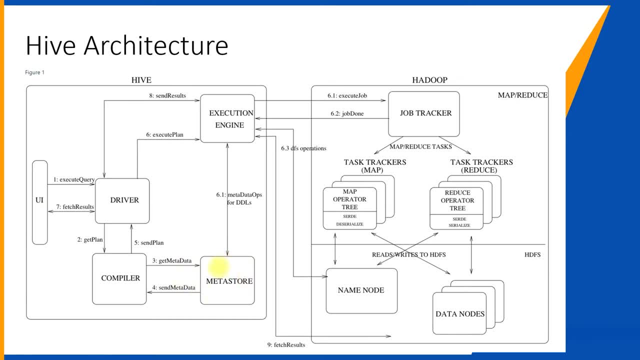 you can see here that we have a meta data about hive itself. so, for example, your tables, column names and where is this, you know, located, what table has what column, so all those kind of meta store, a metadata about hive is actually stored in Metastore. right, this is forced to do it on a MySQL instance or any. 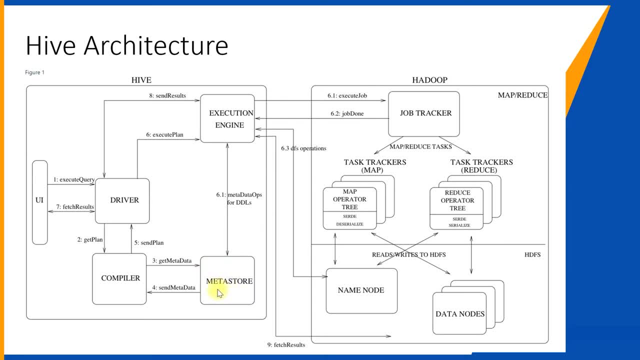 relational database right. this is nothing but a relational database that contains metadata about entire hive right. so that is used for compiling your input, your queries, and then it will send the plan for the driver. once the driver has the plan information from the compiler, the execution is then sent to execution. 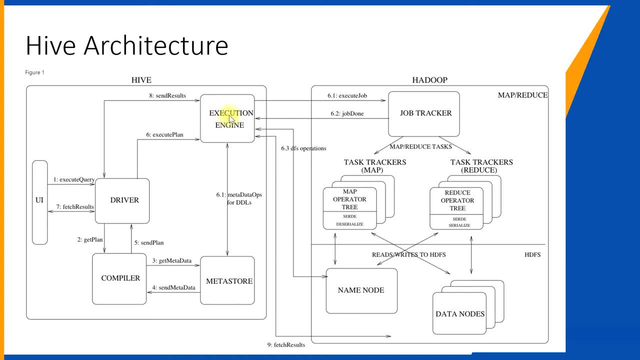 engine. this is also called as hive execution engine. it can be running on, you know, MapReduce or Tez, right, so these are the execution engine. so what execution engine does is it takes the execute plan and it passes the control to the job tracker. so the job tracker is when it will internally work with the Hadoop environment. 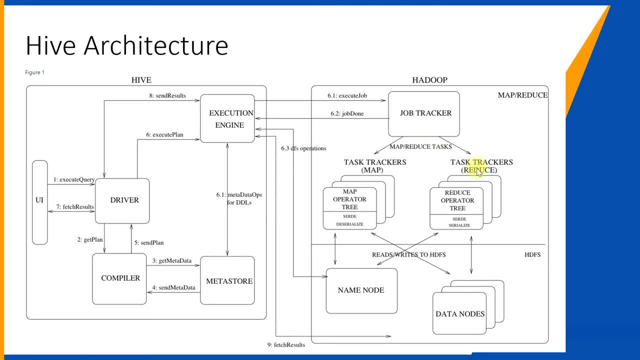 right. it basically spins up for the map and reduce you know tasks so that will internally work with the name node and data nodes. so what happens? when you, let's say, write a select star from a table, the control is passed to the driver, it goes to the compiler, gets all the schema details from the Metastore and sends that. 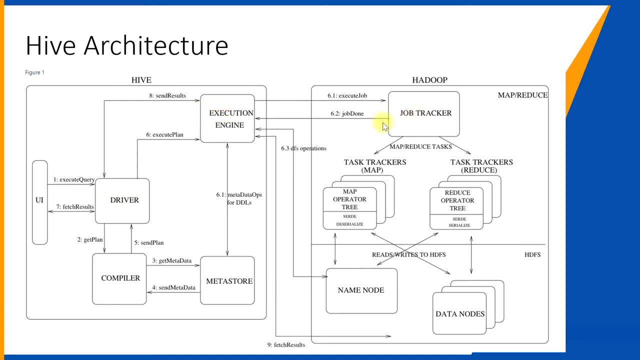 plan to execution engine so that that way, execution engine will communicate with the tracker to get all the data- I mean data from the data nodes- right. so that's how the data- if you look at this last operation- this is how a data fetch is, you know- performed right. so this is all about hive architecture in a very 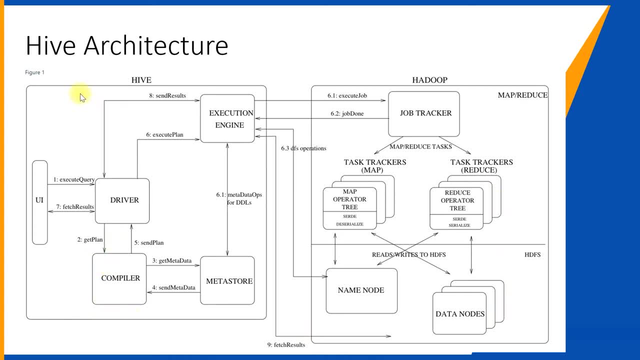 quick session. I know it is a lot to discuss here, but for the sake of you know, wrapping it up early, right, I have got this architecture, so you may want to pause this video and then look at the sequence of activities, how it is performed, and based on that you can have you know better. 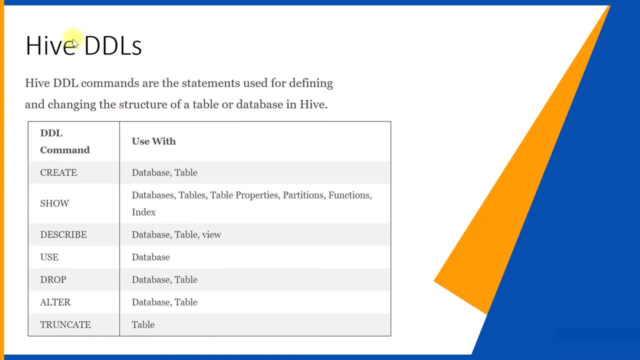 understanding. so let's move on. we will look at the hive DDLs. so DDLs are nothing but data definition languages. so data definition languages are something that you use it for defining or changing the structure of the table or a database in hive. so let's say, if you want to create a new database, you make use of this. create DDL, right, if you want. 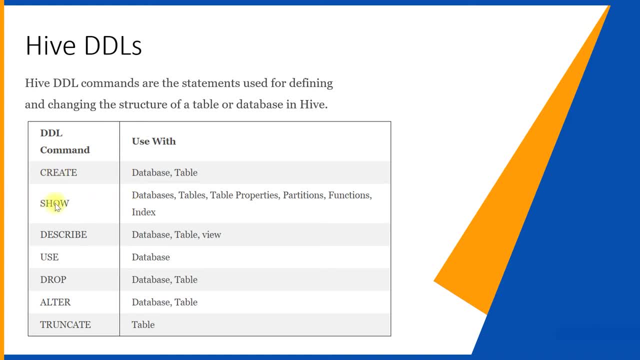 to show. if you want to see, like, what are the tables, what are the database exists, you make use of show a DDL. similarly, you describe to view the content of the table. right, just the structure of the table. describe will give you only the structure of the table and use will actually. 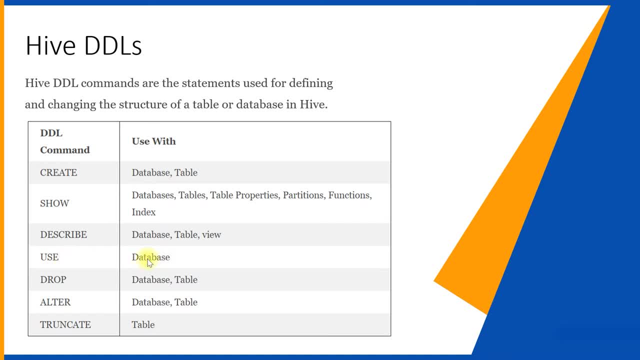 use the database, which means you are connecting to a particular database and then you perform more tables or you know, create tables those sort of you know DDL and using create, you can even create a database or create table or a view, and there are several things I will be looking at. you know. 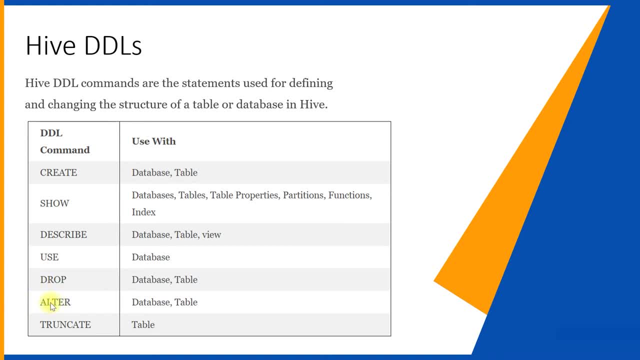 in our hands-on session. we can also perform the alter operations in hive to alter a database and also a table to add more columns or interchange the data type and things like that. and the last one is the truncate. this is to clear the content of the table right, this is the truncate one. so 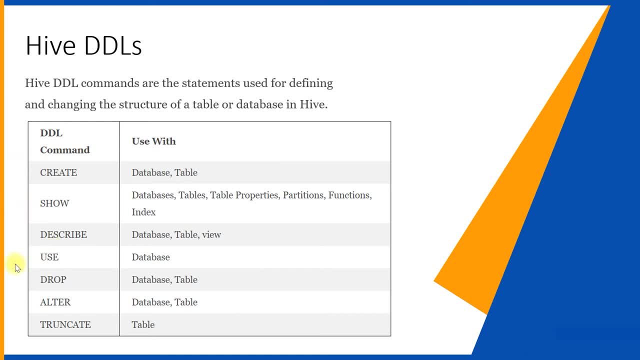 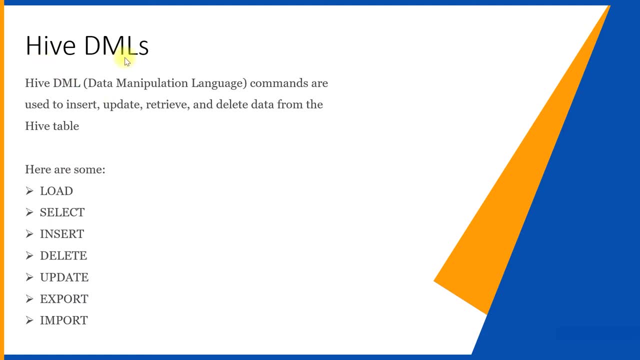 these are some of the hive DDLs: create, show, describe, use, drop, alter and truncate. so moving on, we have got hive DMLs. so DMLs are nothing but data manipulation language. right, these are used to, let's say, you want to insert data into a table. if you want to modify some of the data, if, 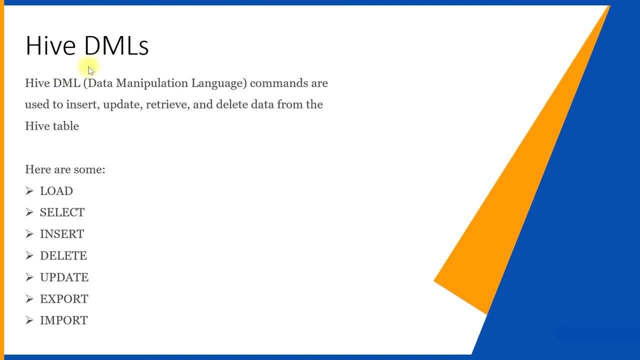 you want to create some of the data. so that's where DMLs come in handy to perform various operations. this, I know most of most percentage. compared to any Oracle or sequel, these commands are very much similar. however, there are few extra options here to specify some of the HDFS related parameters. 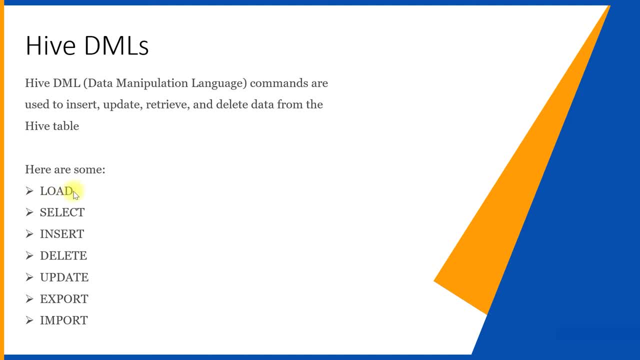 right. so load is nothing but loading your local HDFS path data into hive database. so that's why we use a load local. in path command and, as you might be very familiar, select is possible, select star or select columns from a particular table, and similarly you can insert data, delete data, update data and also you can perform export and 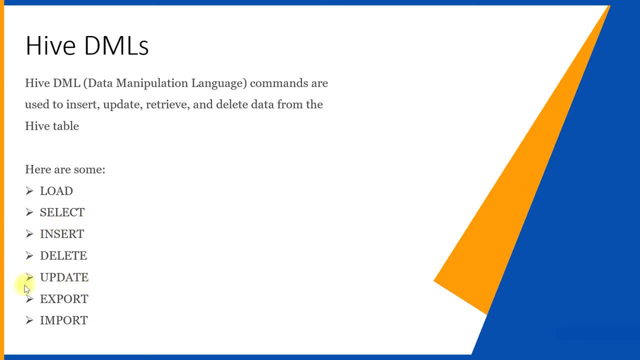 import and, as you see, a initial version of the hive- it was not supporting insert, delete, update operation. these are all you know: asset transactions right. so recently- not very recently, it's been like a few years already- hive supports inserting data- sorry- update and delete is also allowed. 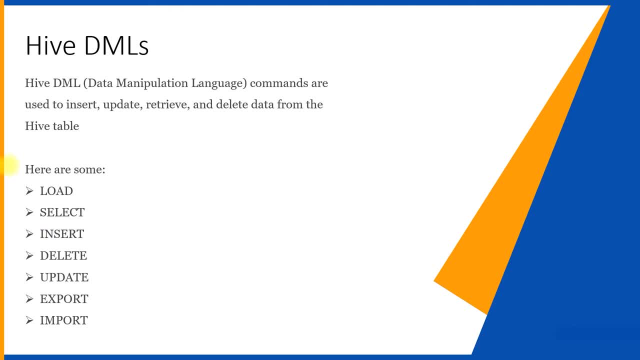 in hive database, but most likely we would not be using update and delete because it's going to be really slow. it is as we discussed in the beginning itself. right, hive is meant for online analytical processing. right, you know you write once, but you read it many times, so that that's. 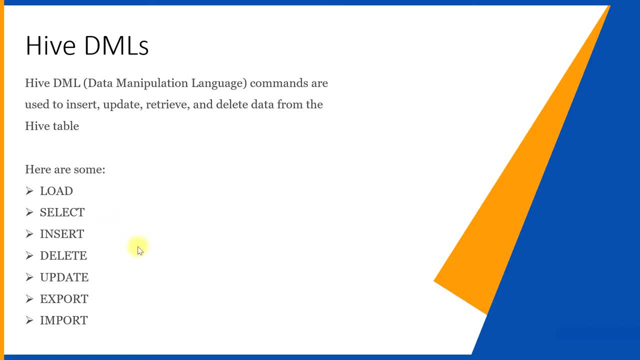 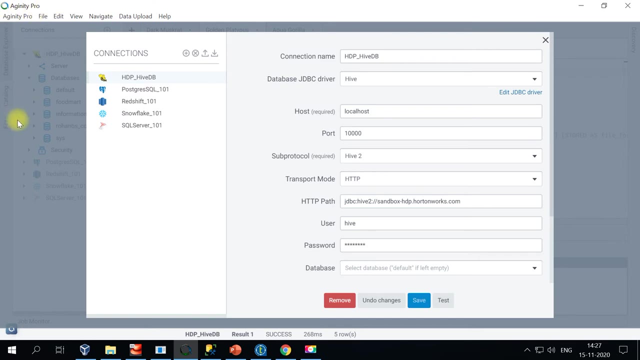 why we call it as overlap. hive is suitable for all app, all right, so let's look at the hands-on. so for that I got a client installed. the name of the client is called agility Pro. this becomes really handy. so it is very easy to you know interact with the hive database, not only hive. 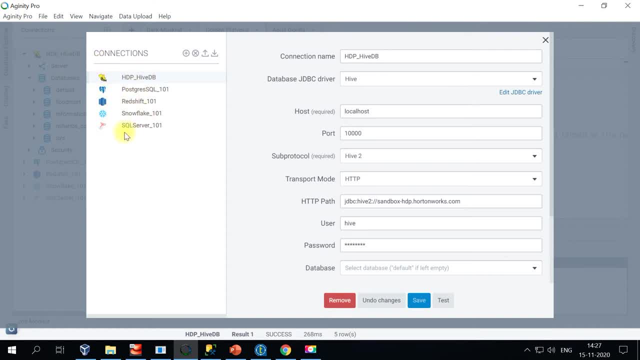 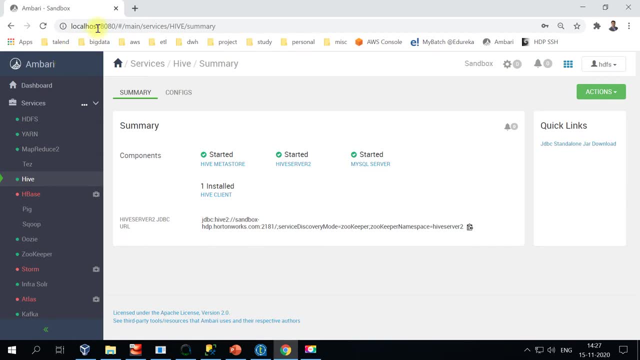 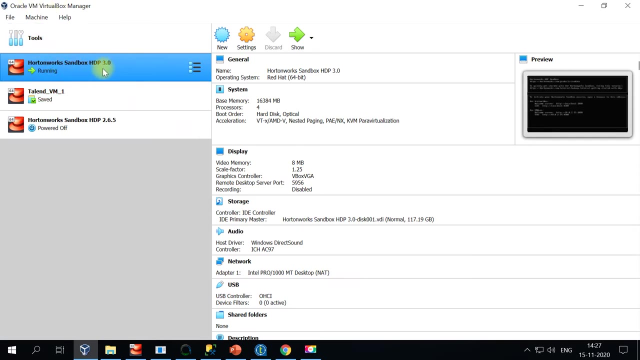 but it supports many other databases, right? so let's um you know before we make the connection. let's look at Ambari here. so I have this Hortonworks sandbox installed on my local computer, so I'm using the Oracle Virtual Box, right? so the Hadoop sandbox is of 3.1, sorry, 3.0, and I have already started it. 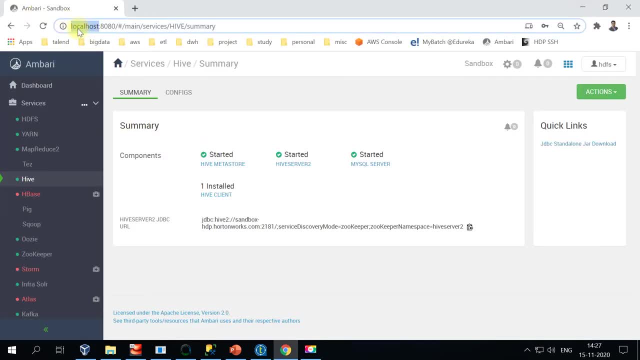 um, so when you uh on the browser, when you log on to localhost 8080 port, it is by default you will be getting redirected to Ambari login page. let me sign out and show it you. so this is how you will be getting a initial screen. 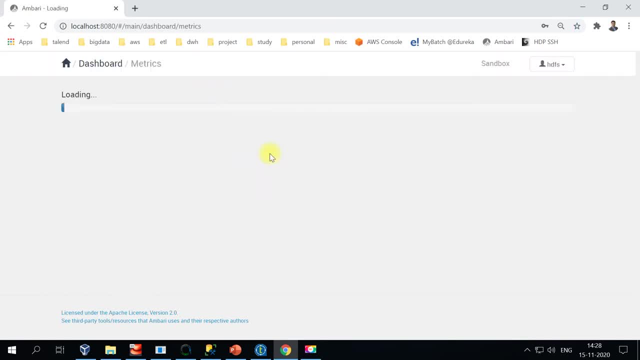 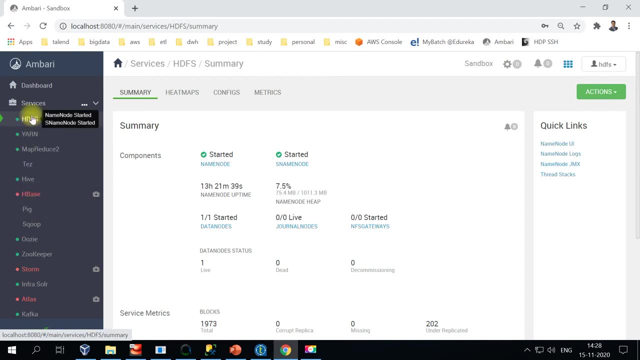 you can use your admin credentials or any other credentials to log into Ambari. when you log into Ambari, you will, on the left hand side, you will see HDFS right. it gives all the information about your data nodes- uh, your name node, if, whether, if it is up and running. if there are any issues, it's gonna, you know, show us here in the 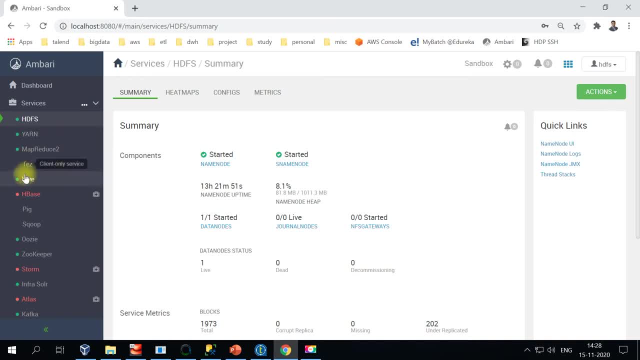 notification, right. so this is all about HDFS. and similarly, you will have a tab called hive. so here, this is where you will see whether my meta store- right, you know that this is where all the definitions are saved- right, the. this is how it stores and shows here in Ambari it will also give: 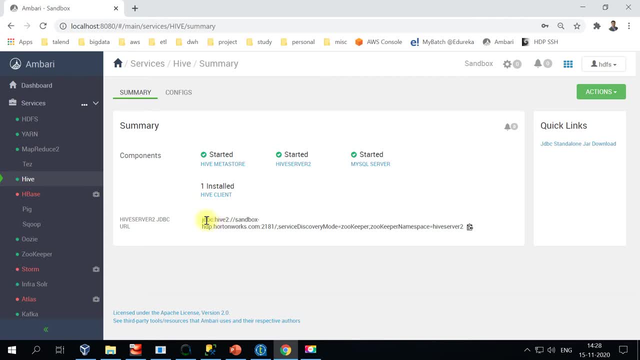 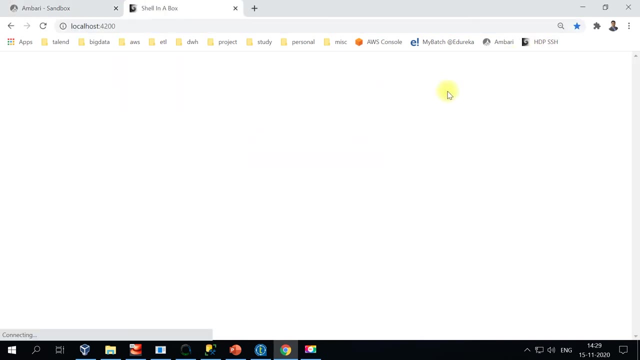 you the JDBC URL for the connections, so you can use it this way: just take this part and then use it on the client right by default. it will also have a high client, but it's not very user friendly. you can even access hive database using a regular, you know, ssh right by logging into hive account and then query directly on the ssh. 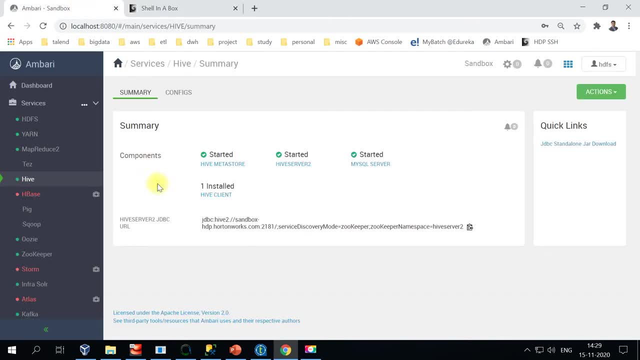 but it's not very user friendly. so we always go with some external, you know, sql client, uh, for some reason, if you have the hive database, you know, installed, but if it's not running, uh, you can go to actions and then start or stop or restart, right. so these are. 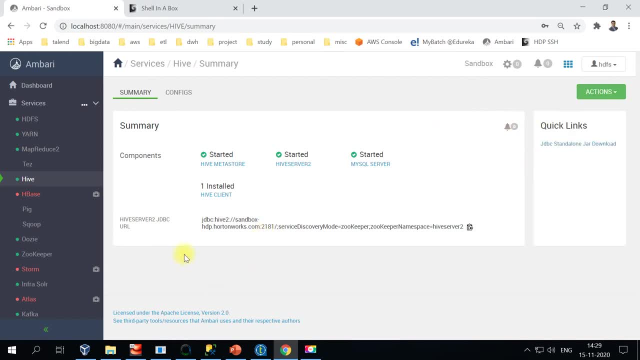 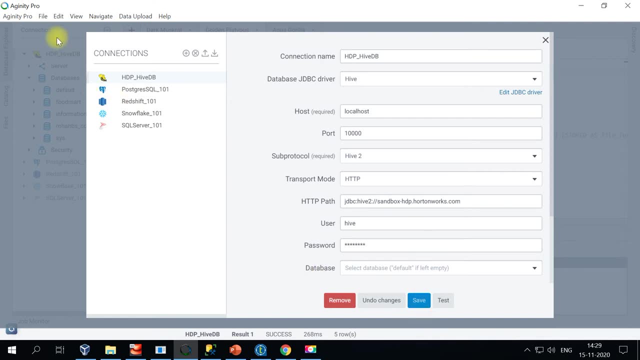 some of the um you know options available, uh, in Ambari. okay, so now that we have looked at Ambari, um, so this is the connection. uh, when you open, uh, the Agility Pro, we can create connection here with this plus sign and, uh, basically the very first time it will ask you to download the driver, right, remember architecture. 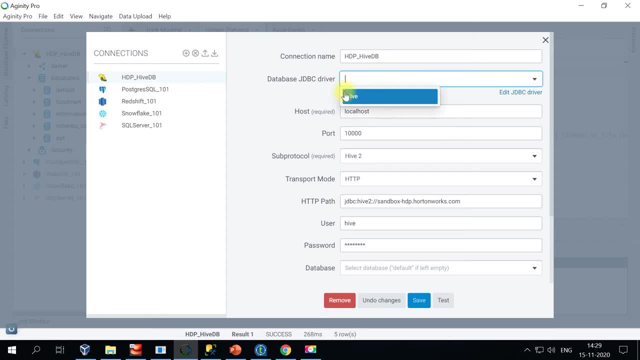 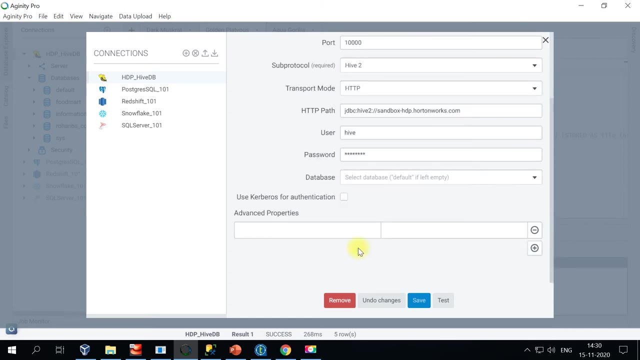 has a driver component, so it lets you download the type driver first, and after that you can specify the local host and standard default port right hive server 2, and you just give the username and you know password if it is set. if not, you can just leave it blank and you can click on test now. 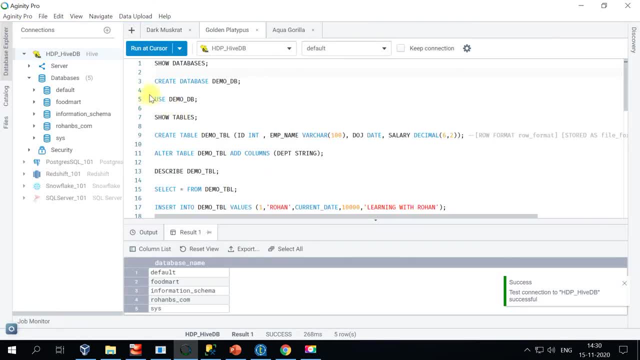 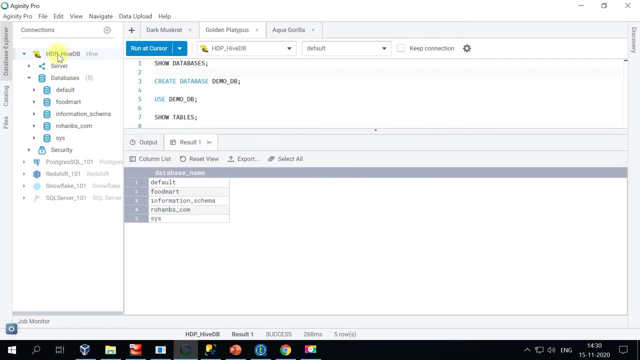 it is successful. right, so now I connected to our database. let's look at, uh, some of the uh DDLs first, right, um, so as soon as you connect, uh, you have a way to choose your database. uh, here, by default, uh, this will be picked up or default will be picked up. and let's see, uh, what are the different. 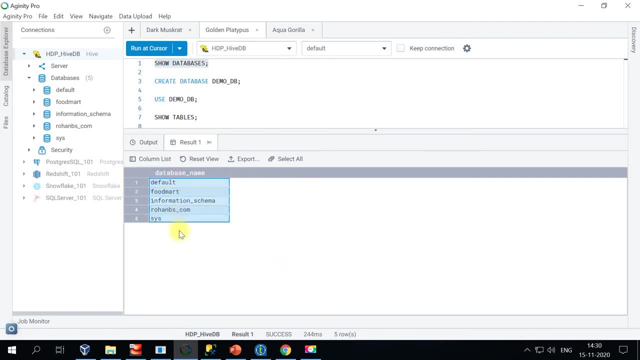 databases available, right? so this lists out all the various database that are available in hive, right? so let's look at the create database command. right? all you have to do is create database and then the database name. okay, so now, uh, the database is created. let's see if it is getting showed up here. 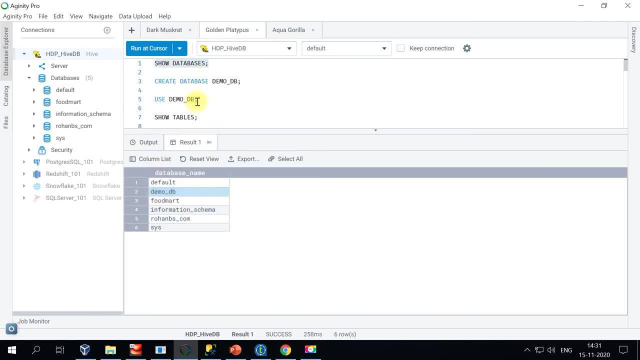 yes, it is demo DB. this is the database that we created. let's make use of that database so, which means we are connected to this particular database, and in that database, let's see if we have any table. because we just created the database, there will not any table, right, um? so when we scroll down, i already, you know, written all this: um ddls here. 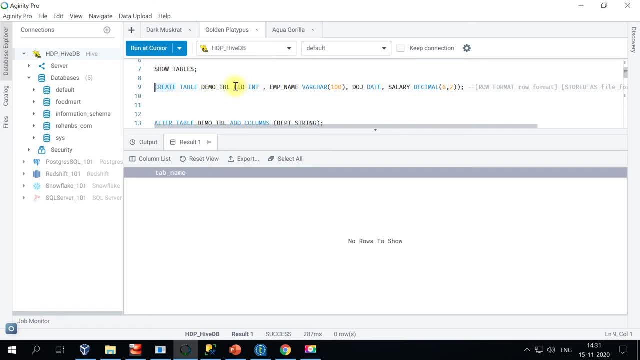 to save some time. so, if you look at it, uh, the ddl for hive is exactly same as, um, you know, regular oracle or sql, but uh, there is an exception here you may want to see and also you may want to pay attention to. uh, the data types. the syntax is: create table, table name, and then the column and 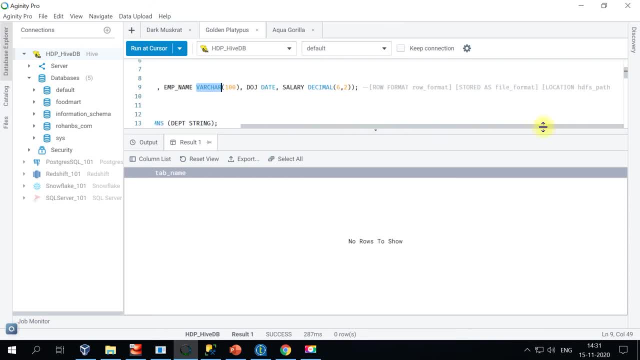 then the data type, right and towards the end you can see these are the optional um parameters for creating any table, so you can specify your row format right. you can even uh specify the stored- as you know- file format, like if you want to do it, as in a csv or txt or zzip or any other type you. 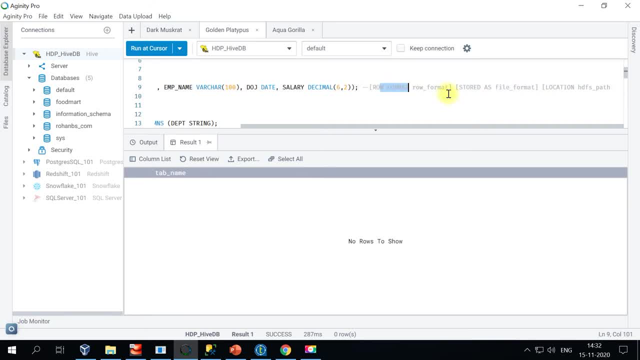 can specify that and uh, for the row format is nothing but delimited. or you know any other format and you can even specify the location. so let's say, if you have the hdfs, uh the file, your data file is already in hdfs. you can specify the location of this hdfs file, so that way it is uh by default, it will. 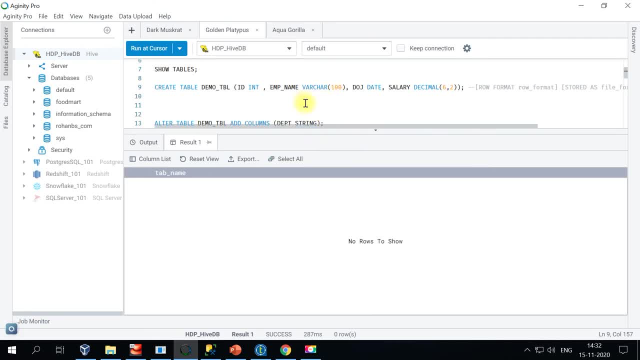 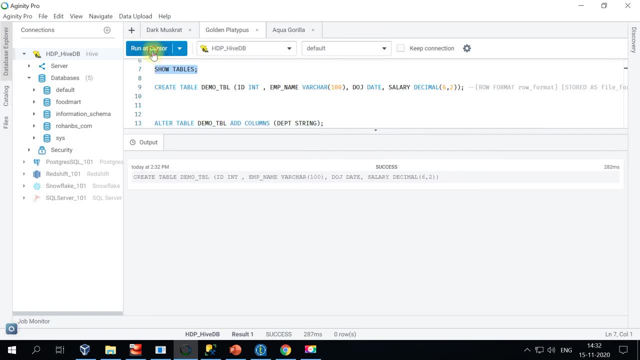 created. so let's see uh show tables now. okay, so now we can see demo. underscore table is now existing. so in order to uh alter, right, you know, we want to see this example also, so you can just keep your cursor and then click on run query. so now uh. 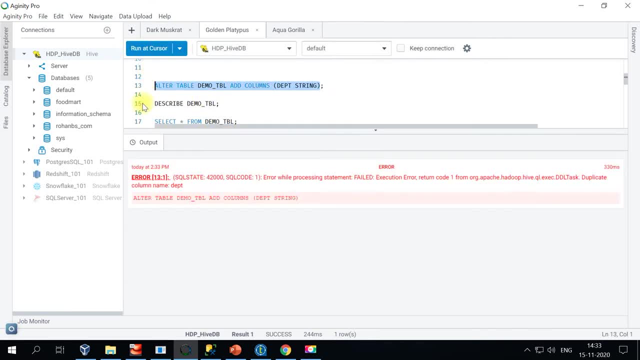 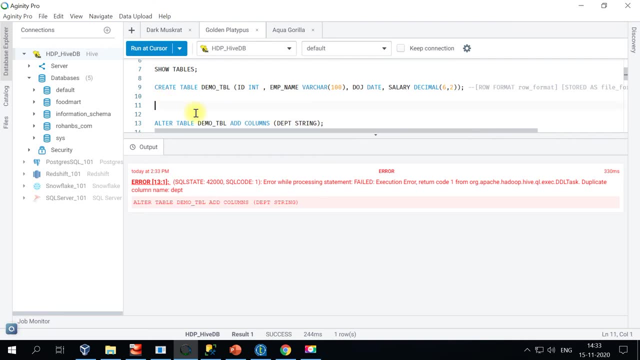 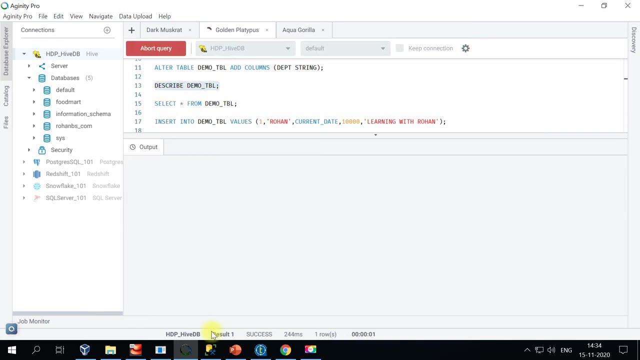 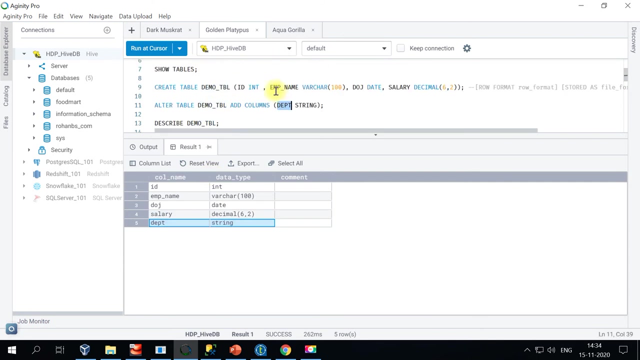 sorry, you can run this command and you can have it. looks like when I executed previously it also executed the alter command. let's see. with describe table, we should be able to see: yeah, so the column is already altered. right, the table is altered by adding this particular column, right? so this is how the describe works. 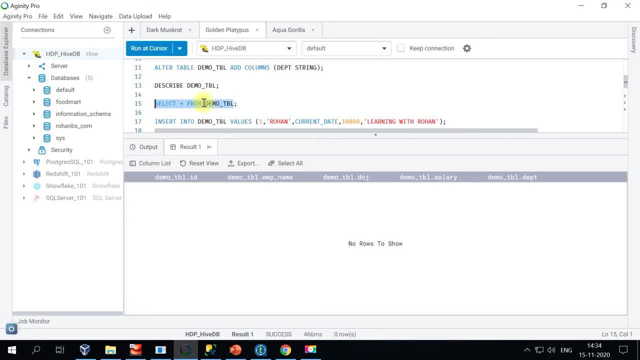 and once this is done you can do a select star from the table name so it will show all the records that are existing. so these are the above ones we have seen as a DDLs right. we also have a few more DDLs towards the end to 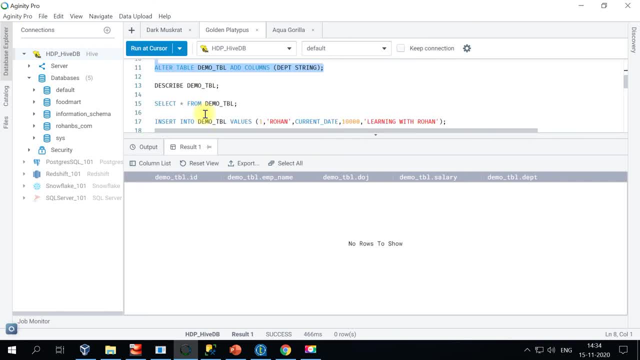 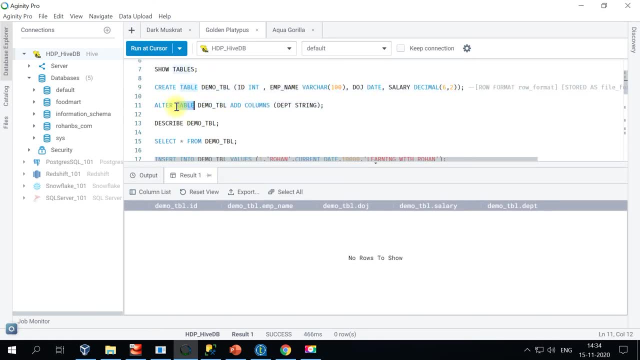 drop the table and drop the table right. so now that we have created a database and a table right, we were now able to alter the table. so now we have created a database and a table right, we were now able to alter the table right. let's look at inserting a data, because our table is right now empty. so 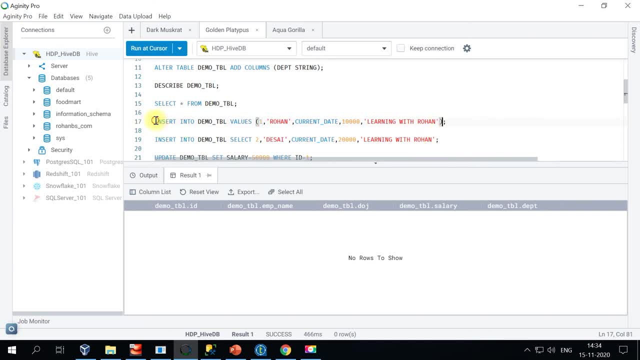 let's look at how do we insert data into a hive table. okay, so now? so let's look at this: insert into a table name and then the values. so the value should contain all the columns that are existing in the table right in the. in our case, we have this ID name and the date, salary, and. 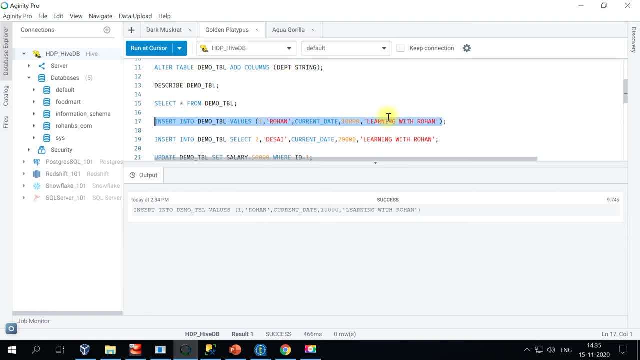 then the description- sorry department- of this particular record. now you see the record is already inserted, right. so this is one way of you know hard coding your values and then inserting the data. so there is another way: you can even write your select query and then insert your data into hive, right. so for that we will. 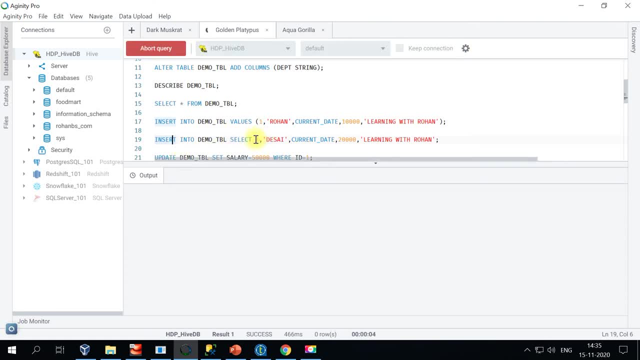 be writing: insert into table name, select, and then that all the columns- if we are actually- I mean if we are heading towards our current table- we will, of course, har Tet this way every day. now we'll see how that works, because if any of the column is missing, then the query will not work and the data will not be. 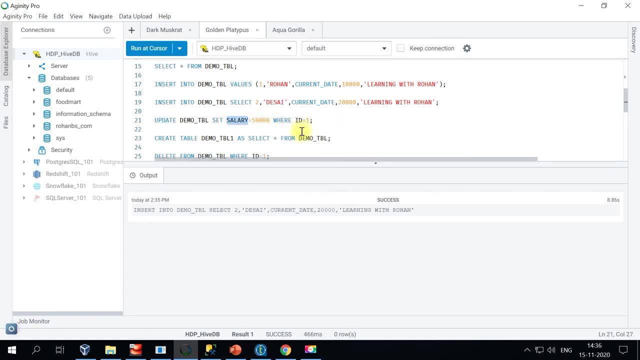 inserted. okay, so this is how it works, and now I topo from some update. what I'm going to do is I am going to use one of the column called salary. right, I'll be using this column called salary and I want to change the salary for this. okay, so often, some things you can do is have your table. 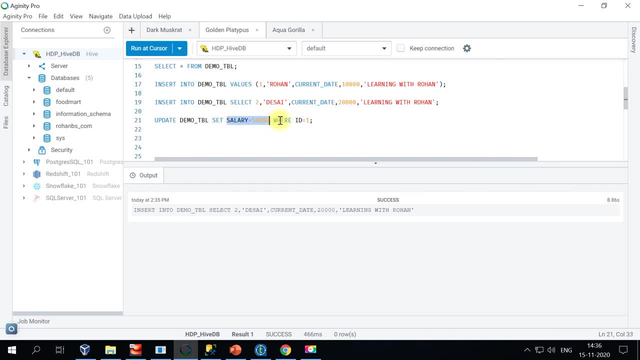 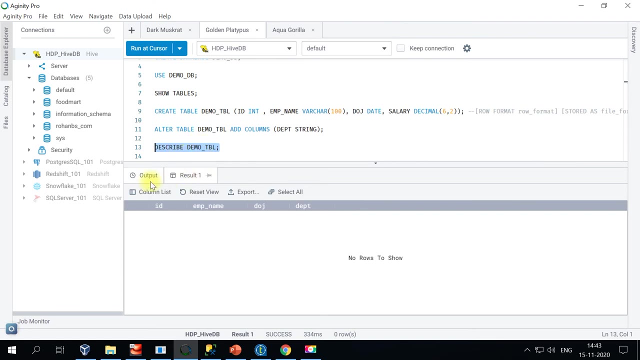 set salary equals to so-and-so where the ID is one, so only one record. where the ID is equal to one, the salary will be updated. okay, so the describe table name command statement is used to list down all the columns that are existing in a particular table. it will also show the data. 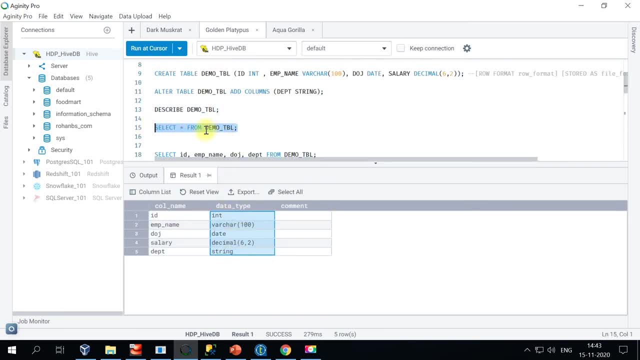 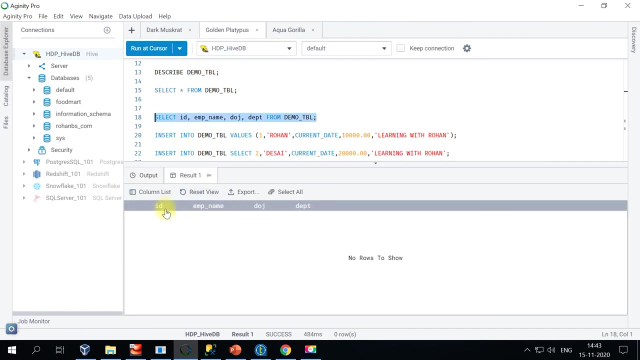 types and moving on, select star from a table will show the data from a particular table. you can do either start to get all the column names or you can even choose a particular columns from a database. okay, so this is how it shows: the column names on the top and the data we don't have. 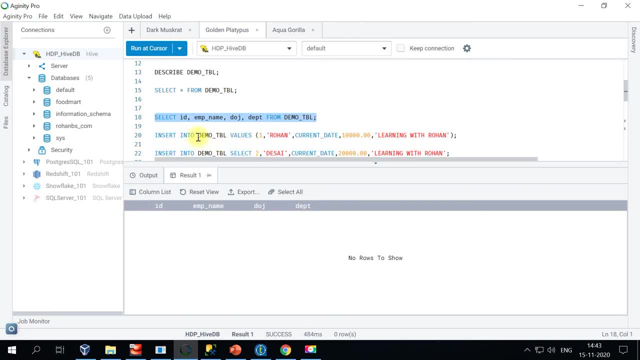 anything now. so let's do a quick insert into this particular table. so here is the insert command: insert into a particular table. so here is the insert command: insert into a particular table name. and then the values. so this way you provide your hard-coded values for whatever columns you. 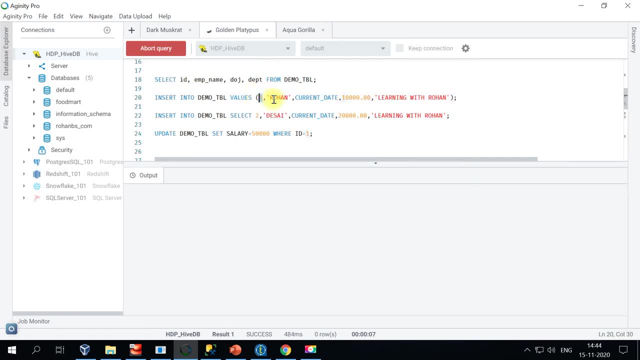 have. you should be providing the values for each and every you know columns for in that particular table. and there is another way. instead of hard-coding values, you can even use a select statement to pick up the data from some other table or any other you know place. you can even. 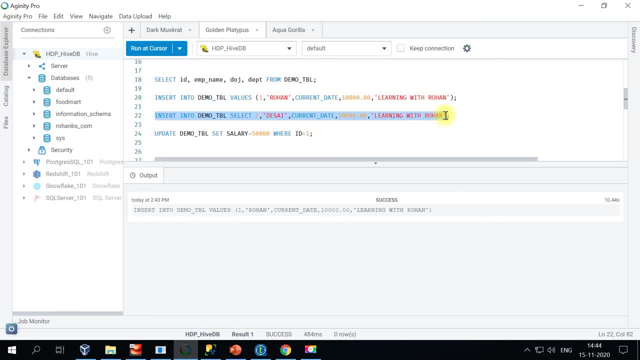 use insert into this table along with select from a different table. you can do that as well. so for now, I just took an example wherein I'm showing select from a hard-coded value, but if you have a table, you can directly get it from there, right? so this is how your insert works. are two types of insert? 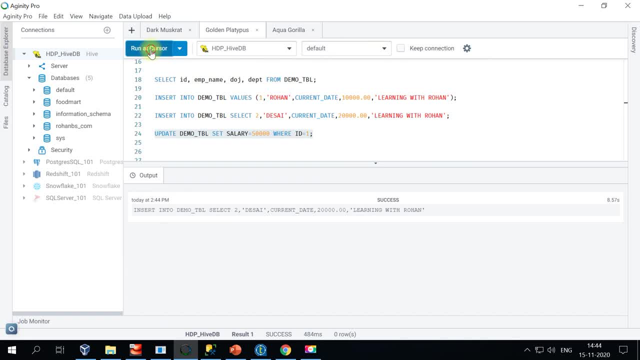 and coming to updates, you can perform any update for a particular column along with any condition, so the syntax is update, table name insert. that's it. so that's all for today. so thanks for watching till the end. I hope this was helpful and if you have any questions, please feel free to write a comment. 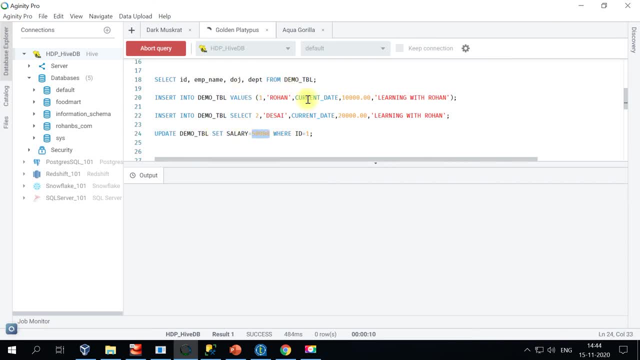 if you have any question, please feel free to write a comment, and so the syntax is: update table name. set the salary or whatever fees that you want to set. you can set the value for that, but we should be giving you know the weight loss as well, so that only. 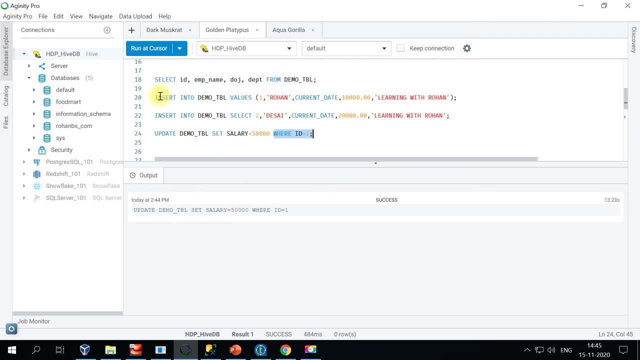 that particular record gets executed. so, as you might have already observed, the insert and update operations are pretty slow in Hive that I'm using my local sandbox. yeah, it's going to be faster with the real, you know, Hadoop notes. right now we have only one node, so it's little bit slower, okay. so now that we 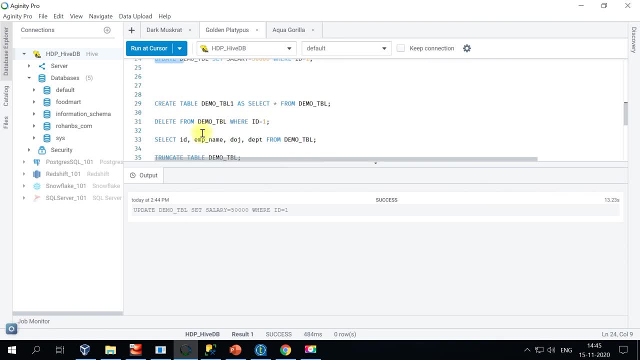 have looked at insert and update. let's look at one more: create command now. so what I'm saying? I'm creating another table by selecting the data from one table, the table that we just inserted data. we will do that operation: create table, demo table one- and select from the existing table. so this will 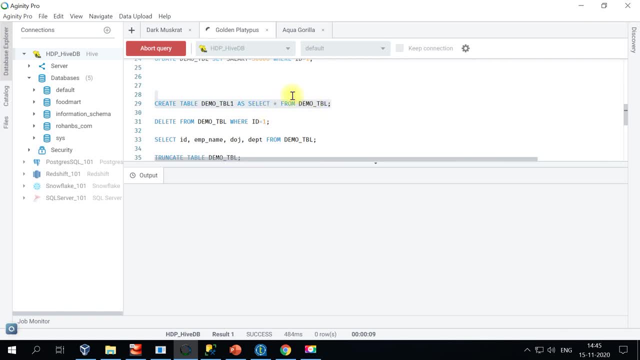 automatically take care of copying the structure and the data from this particular table to your new table. so the new table is now created. so now let's look at a delete operation. the syntax is delete from the table name where the ID equals one right. so let's do that delete and then look at the date. 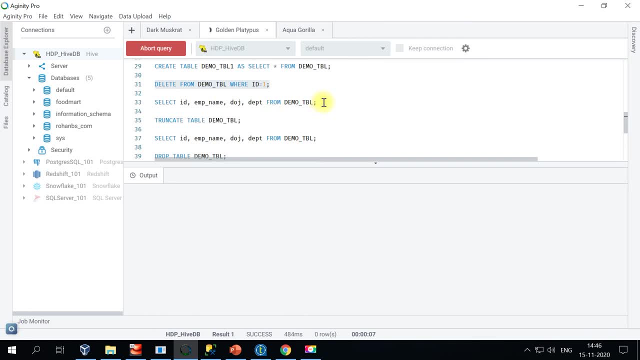 table. if one of the records is taken, we will get a deal deleted. let's go ahead and color, excuse me, yeah, all right. we need to create a new distribution here that hide it, and we have itistened to. we need to create a new distribution here that hide it, and we have itistened to. 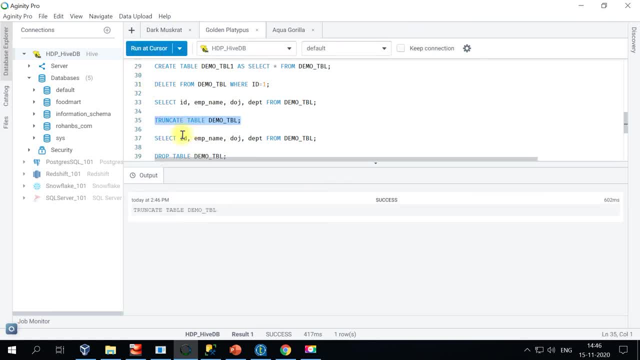 delete and update one of the records as well. delete and update changes between all two devices. now we know the way it's going to work. okay, so that includes Vegas will be deleted. truncate is always faster compared to delete because it's not keeping track of any deletion right. so now, if you do a select star from 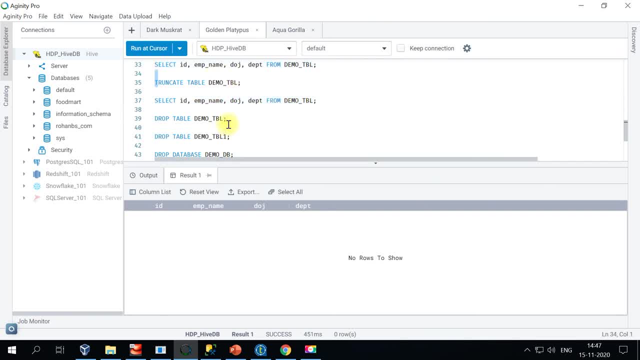 table. the table is empty because we just truncated it. now we'll look at couple more DDL operation, which is drop table. so we created this table, so I'm gonna drop that. so the table is dropped and let's drop the other table also that we created right. so before we do that, the final drop database. if you go back and